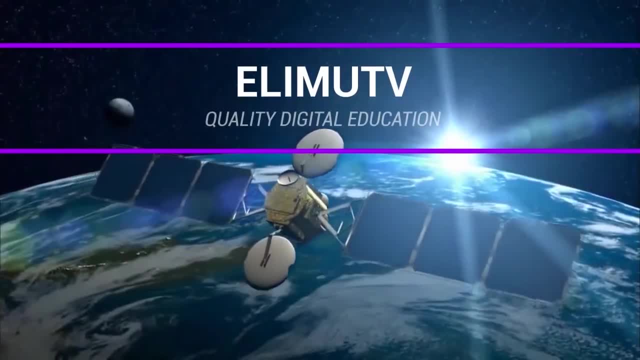 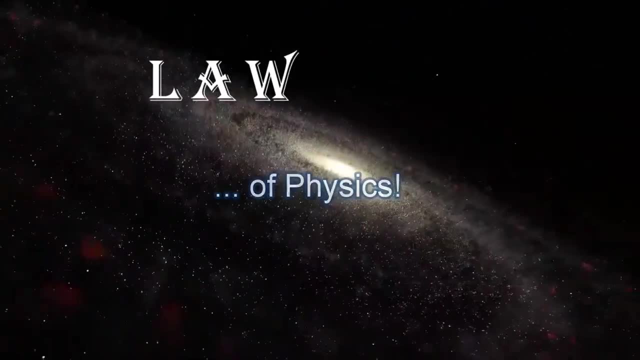 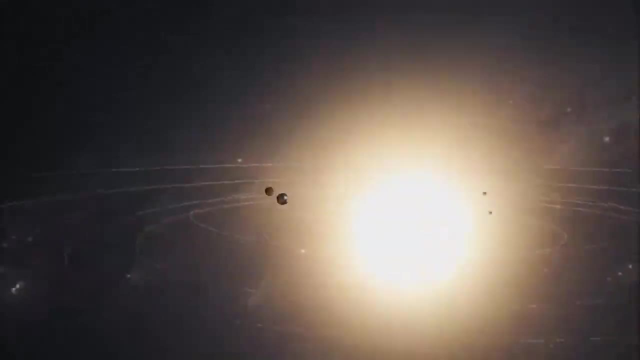 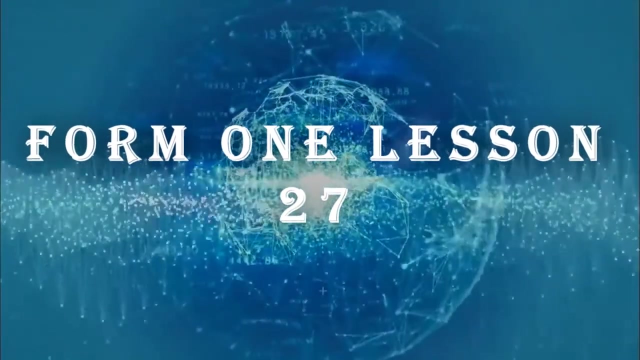 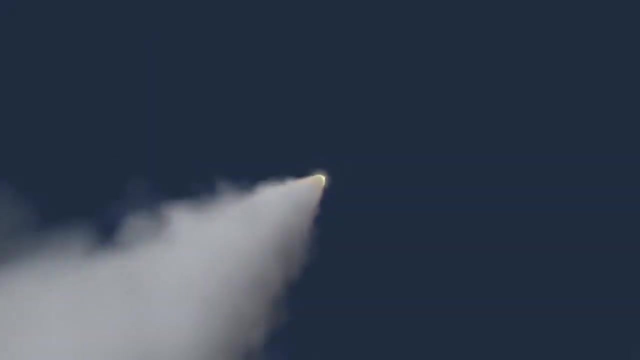 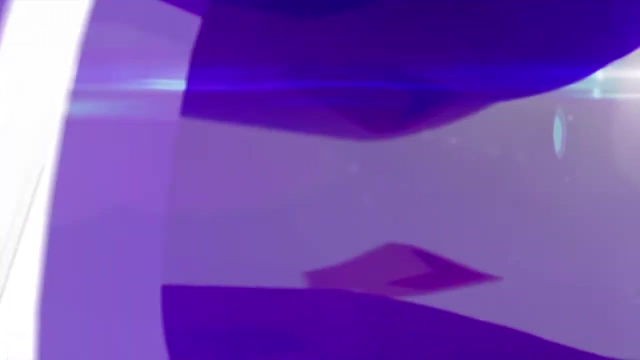 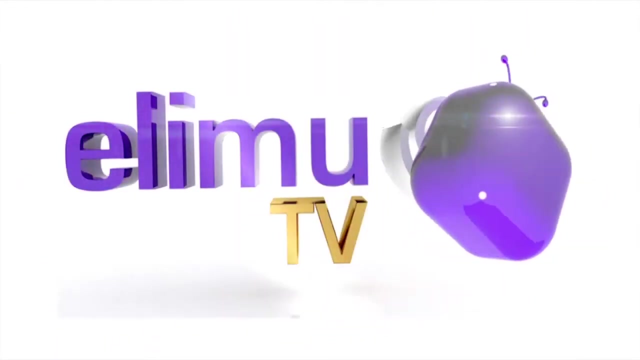 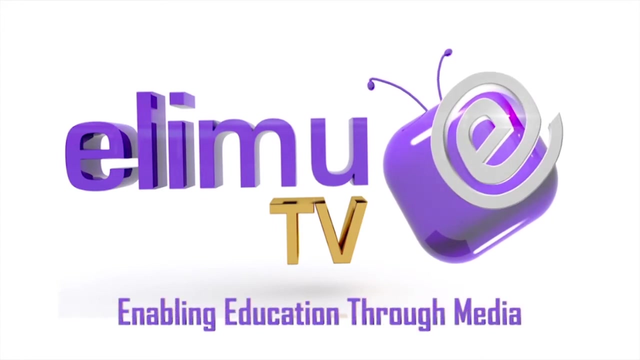 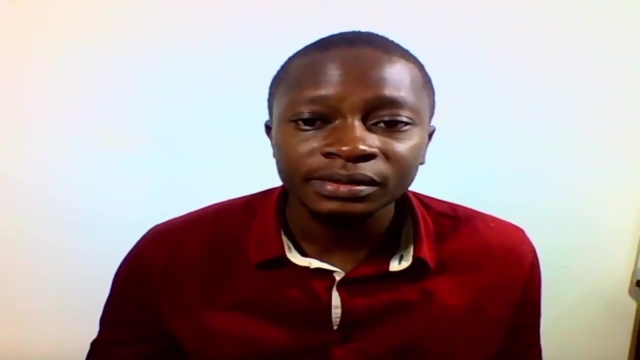 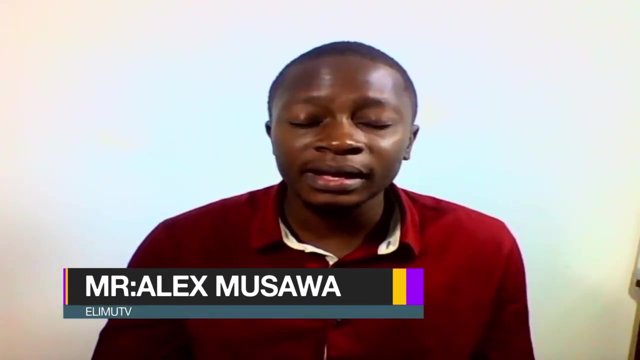 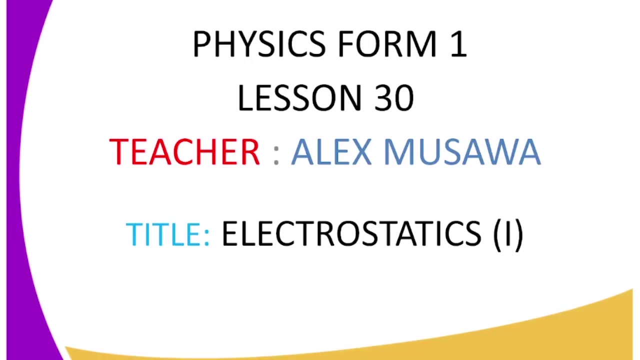 Thank you for watching. Thank you for watching. Welcome to Elimu TV, a place where you watch and learn. I am teacher Alex Musawa and I'll be taking you through Physics, Form 1, lesson number 30.. Our title is Electrostatics 1.. 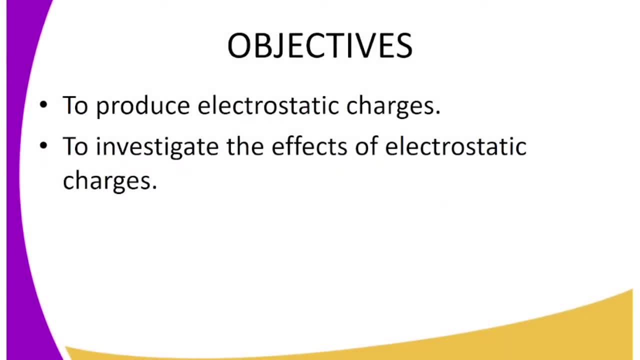 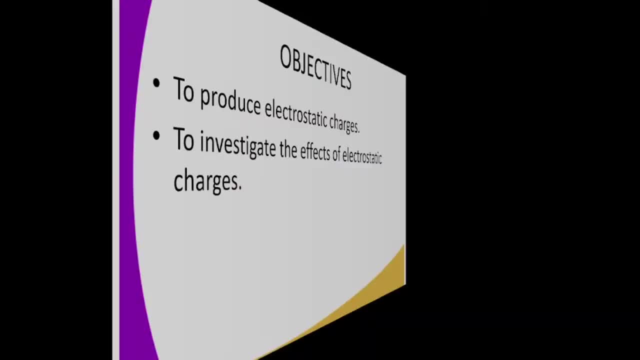 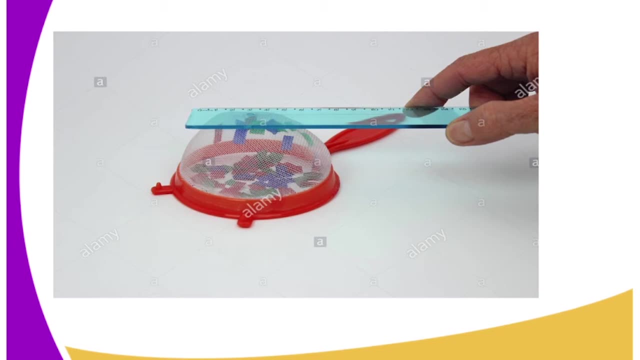 The objectives of this lesson are to produce electrostatic charges. number 2, to investigate the effects of electrostatic charges. And, as you all know, everything has charges. Everything includes the arulla, your cup next there to you. Everything has electrostatic charges. 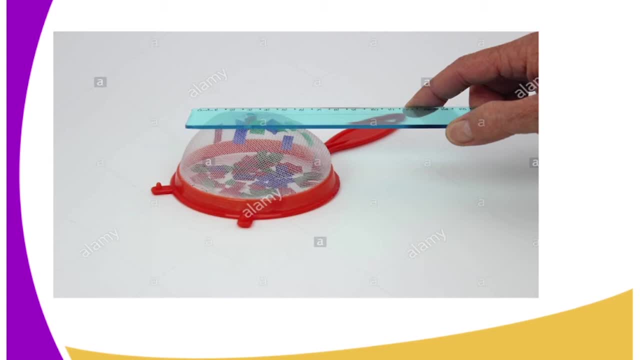 And the reason why they're called electrostatic charges is because these charges are at a point, They are not moving, They are electrostatic, They are induced And, as you can see from the diagram, we have arulla And we have PcT. 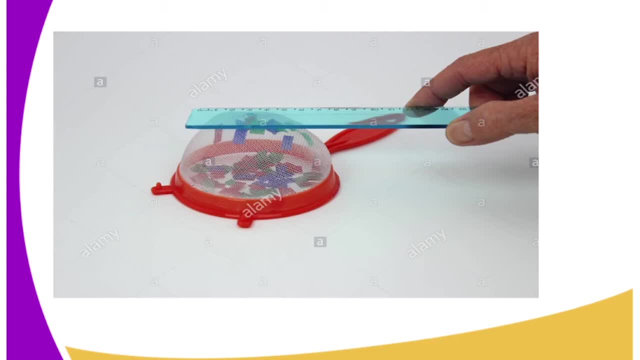 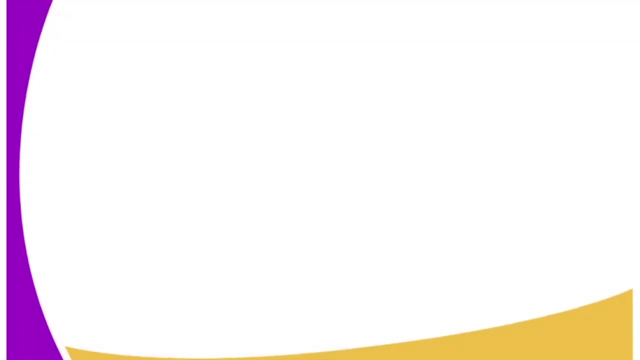 of paper. what happens when you take a ruler and you rub on over your hair and put it close to the pieces of paper? what you see is that these are the something that is happening there: the ruler attracts the, the papers. we have another example with how a balloon, a balloon that has been 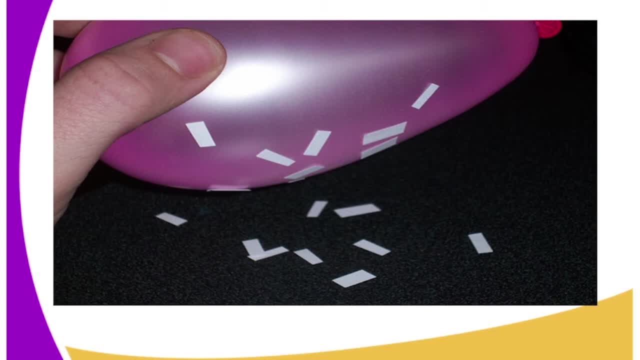 little air and what? what? when you take the balloon and you rub it over surface and then you bring close to the pieces of paper, what happens? the piece of paper are attracted. this proves that electrostatic charges exist and they are induced upon rubbing an object on a surface. 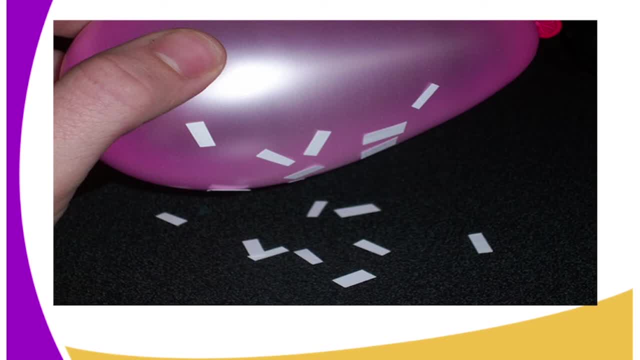 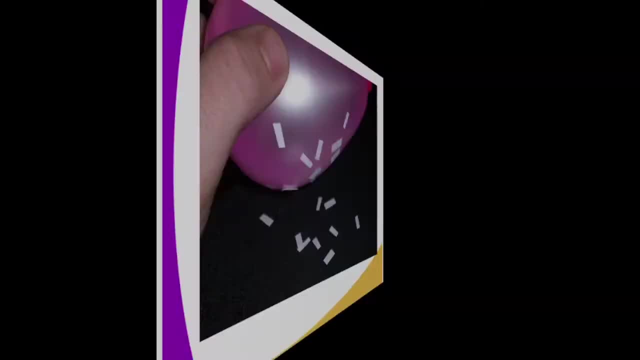 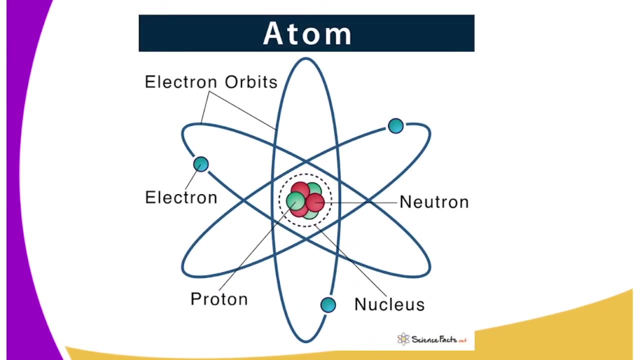 as you can see there, the balloon that has been rubbed over surface. we have induced some charges that have been able to attract the papers. our next point: so where do you think these studies are coming from? as you can see, we have an atom, and an atom is made up of electrons, protons and neutrons. the electrons consist of the positive charge. 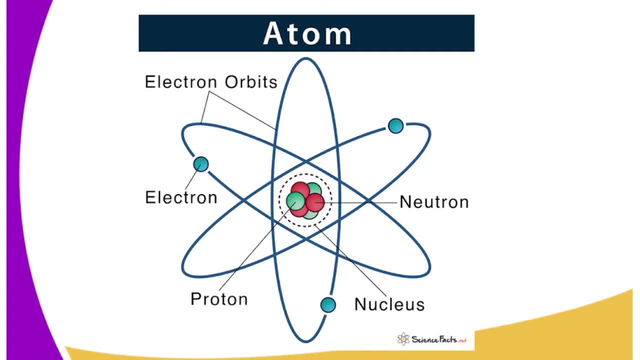 particles, the negative charge particles and the protons, consists of the positively charged particles, the neutrons. they are neutral, they don't have any charge. so where the positive charge of an object, where the coming from from the protons and the negative charge are coming from the 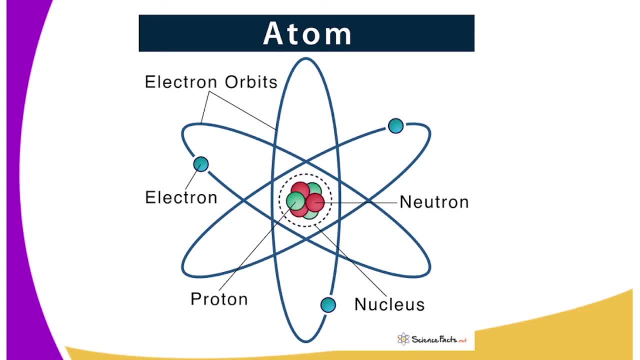 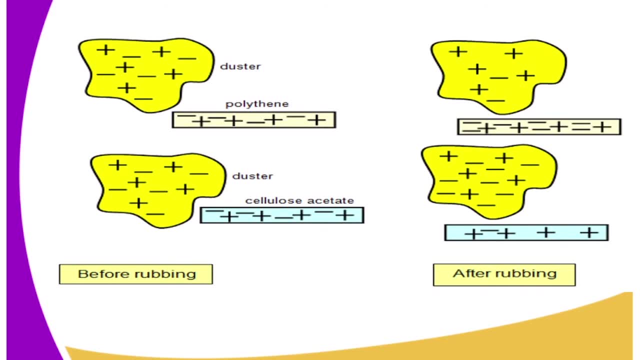 electrons. next point, and that is why, when we take a ruler and we rub it over a surface and bring it close to the pieces of papers, what happens is that the piece of paper they are attracted one is because charges are induced upon rubbing. and if, when, when you see, can you see from it before rubbing the charges? 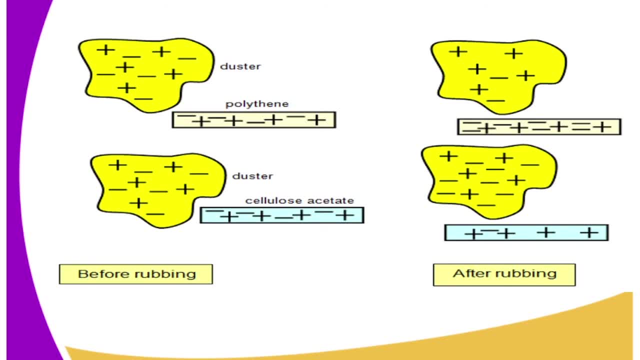 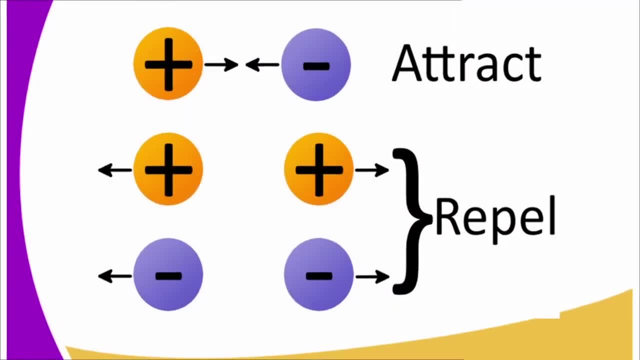 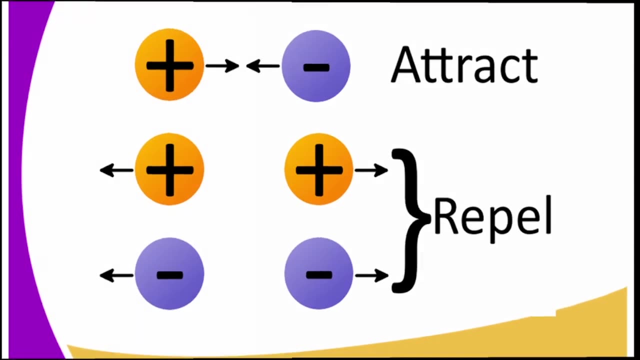 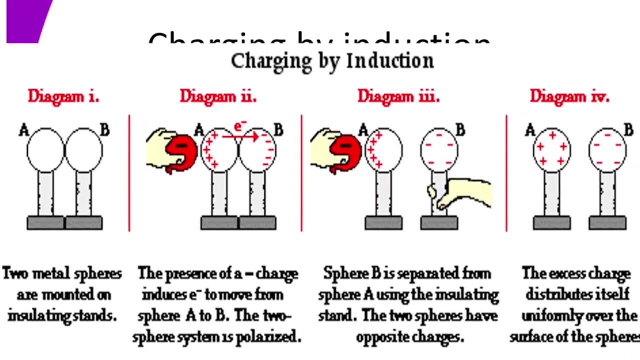 are not distributed. they are not distributed even, but after rubbing the charges become distributed evenly and that causes them to either attract or repel. as you can see the light, charges attract and unlike charges repel. the first is charging by induction. as you can see, there there are two metal. 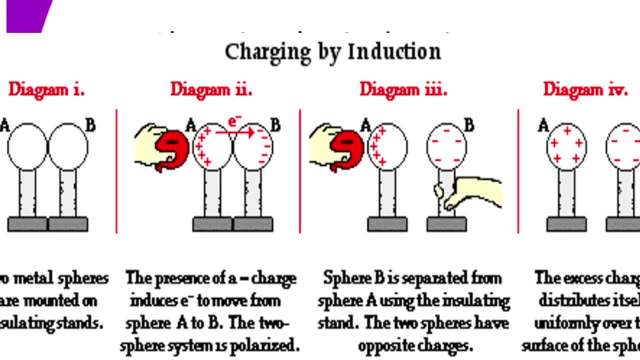 spheres a and B. so we are going to bring a negatively charged sphere close to A and B. what happens? since the positive charged particles are not, they cannot move, they are going to remain at point A, while the negatively charged particles, which are the electrons, they are going to be repelled, because we have seen that and light. 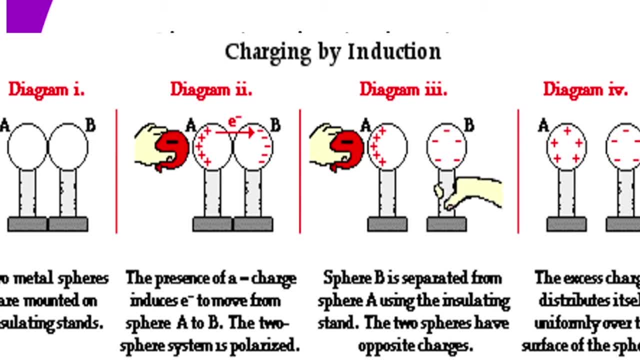 charges repel. they're going to be repelled the far end of of the sphere B, and then we are going to separate the two spheres and then what happens? the charges in A, they are going to be redistribute themselves and we are going to have the positively charged particles in sphere A and in B. we are 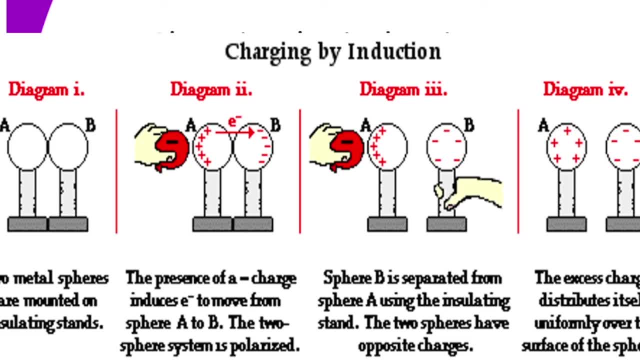 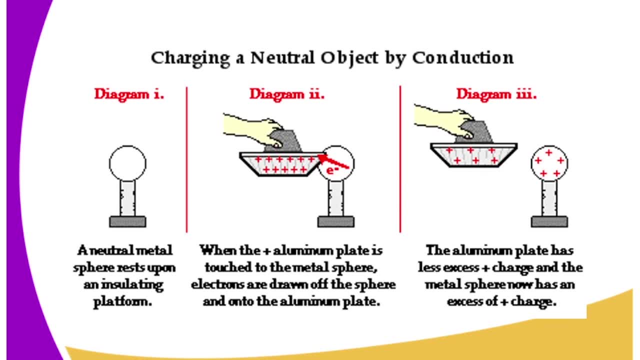 going to have the negatively charged particles. next, we are charging an object by conduction method and in conduction method we have an earthing it's it involves, whereby we are going to earth the electrons from there, from the object. consider the situation there. we have a neutral sphere. so what happens when we 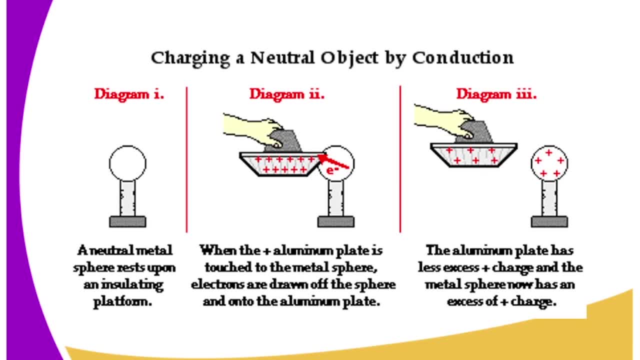 bring up a positively charged object before the sphere and we are going to have an earth and in this case, our earth is going to be a thing is going to be the hand. so the positively charged particles, they are going to attract the negatively charged particles and as they are attracted, since these are called, 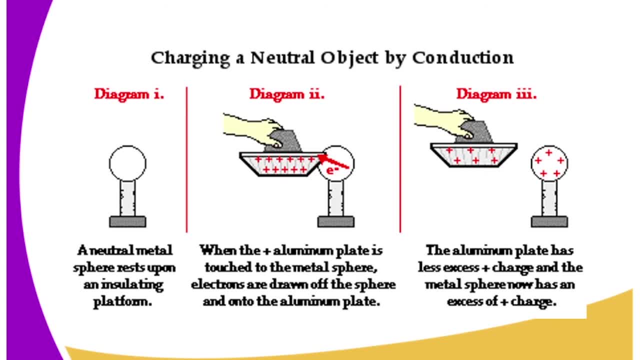 these are contact there. what happens is that a negatively charged particles that we move into the body of the person- many that, and then we separate the two in the negative in charge particles have moved away. the sphere remains to be positively charged. and as the charges redistribute themselves, the sphere remains positively charged. one thing you. 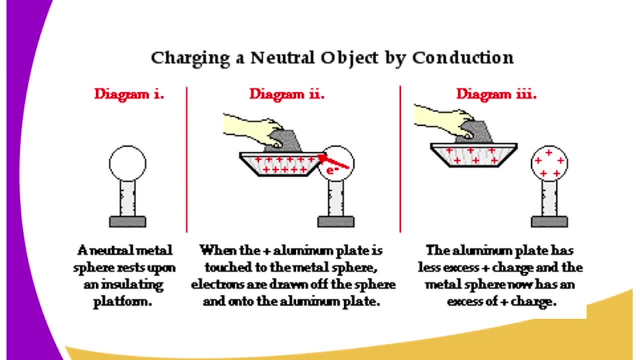 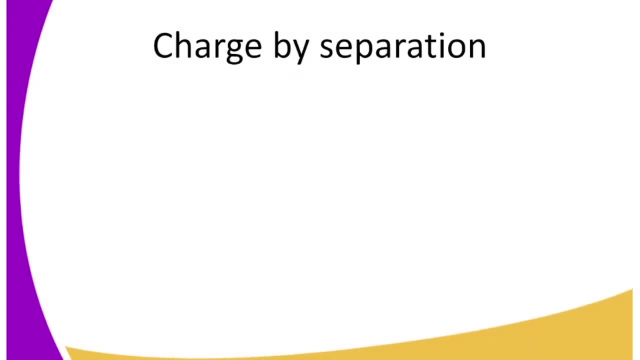 notice when charging an object by conduction is that the object takes the charge of the, the object that is trying to induce the charge, so both of them are positively charged. Next we have charging by separation And from our case you can see we 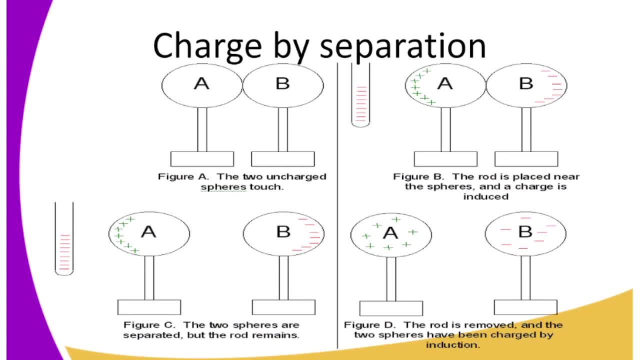 have two spheres there, sphere A and sphere B Two. what happens when we bring a negatively charged object in front of the two spheres? The negatively charged particles? they are going to be repelled by the object to the far end of sphere B, So we have the positively charged particles. 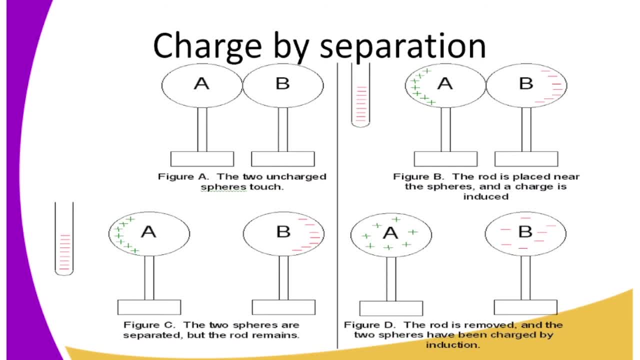 remaining in sphere A, as you can see there. And then when we separate the two, suddenly what happens is that the positively charged particles in sphere A are going to redistribute themselves, And so our sphere A is going to become positively charged, while the negatively 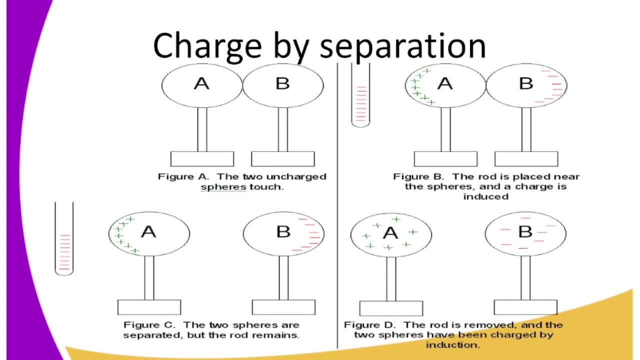 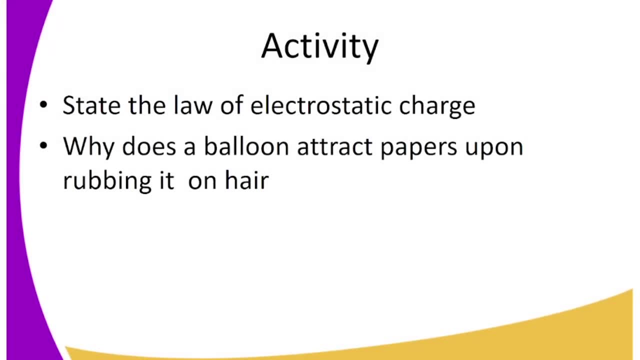 charged particles in sphere B. they are going to redistribute themselves and sphere B becomes negatively charged. And that is the end of our lesson. I have an assignment for you. Number one: set the laws of the universe. Number two: set the laws of electrostatic charge. Number two: why does a balloon attract?